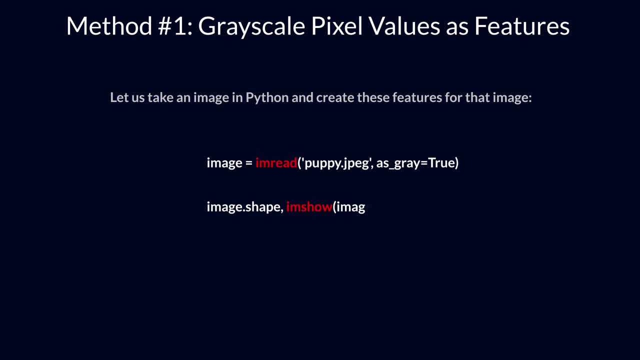 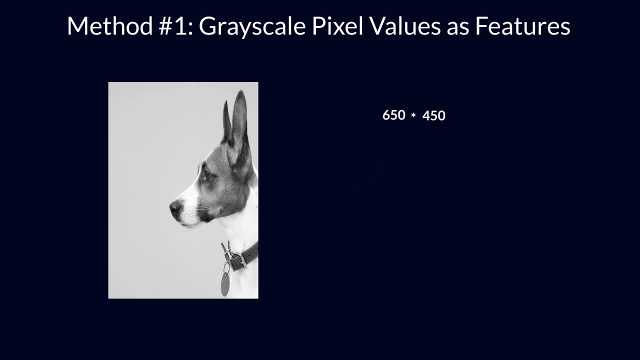 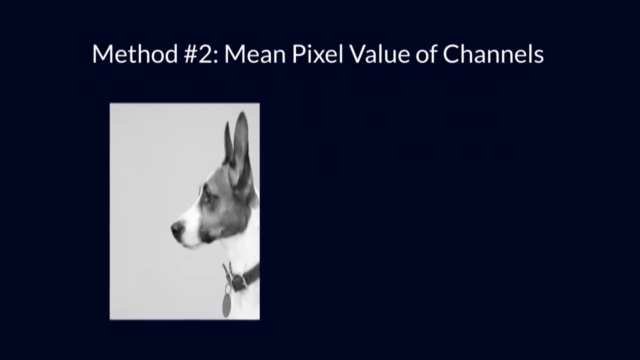 image and image Shape method to get to dimension. The image shape here is 650x450.. Hence the number of features should be 297000.. We can generate this using the reshape function from numpy, where we specify the dimension of the image. Let us move to the second method, called mean pixel value of channels. While reading: 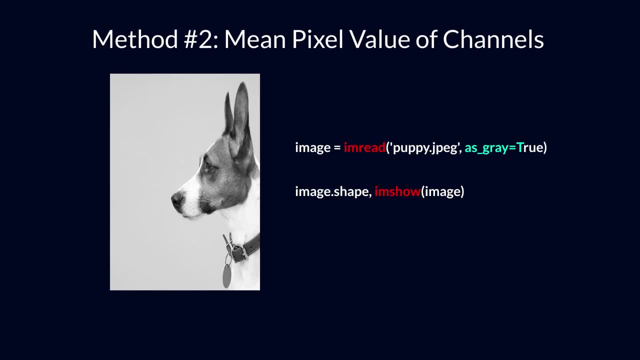 the image. in the previous section we had set the parameter as gray equals true, so we only had one channel in the image. Let us go back to the previous animation and we can easily append the pixel values. Let us remove the parameter and load the image again. This time the image has a dimension. 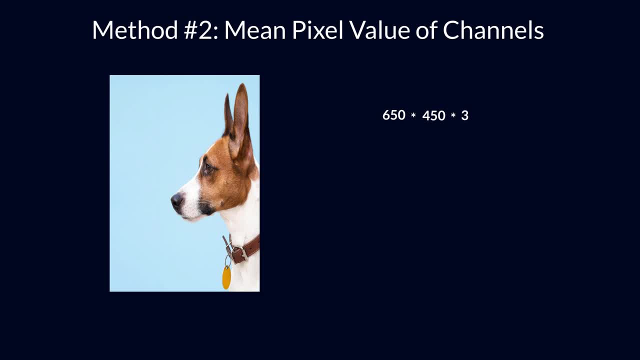 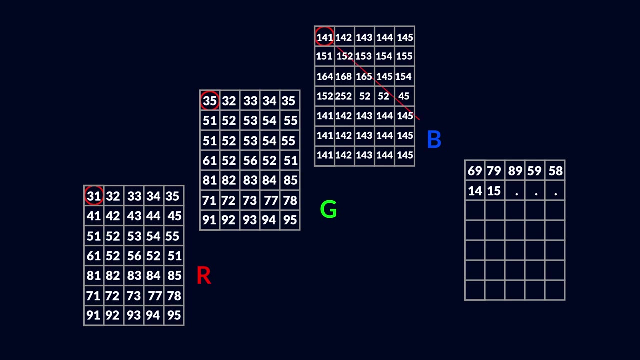 660x450, 3, where 3 is the number of channels. We can go ahead and create the features as we did previously. Instead of using the pixel values from the 3 channels separately, we can generate a new matrix that has the mean value of pixels from all 3 channels Just. 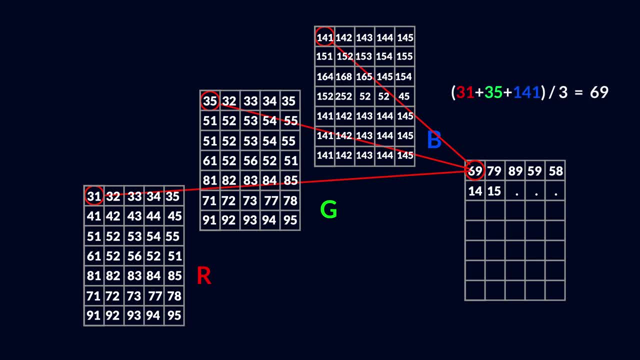 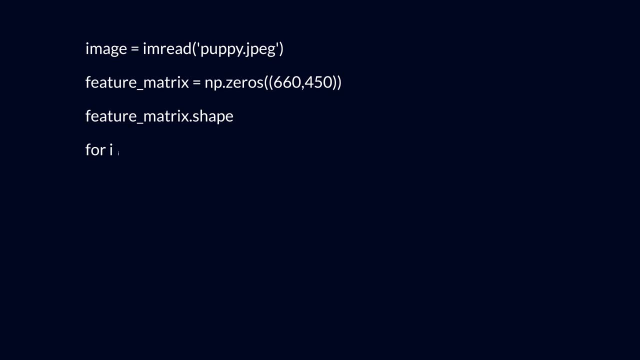 channels. By doing so, the number of features remains the same and we also take into account the pixel values from all three channels of the image. Let us code this out in Python. We will create a new matrix with the same size- 660 x 450, where all values are initialized. 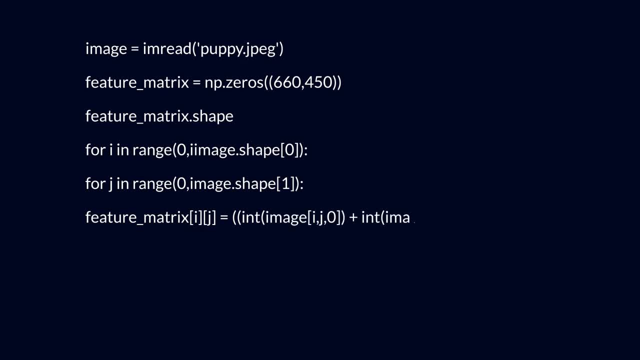 to zero. This matrix will store the mean pixel values for the three channels. We have a 3D matrix of dimension 660 x 450 x 3, where 660 is the height, 450 is the width and 3 is the number of channels. To get the average pixel values we will use a for loop, The 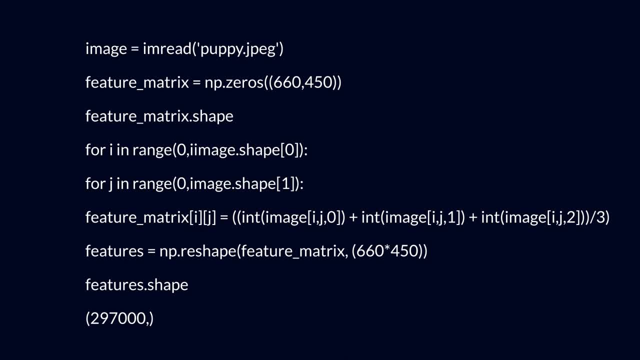 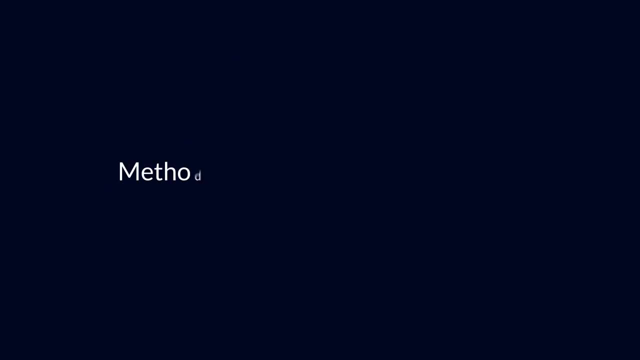 new matrix will have the same height and width, but only one channel. Now we can follow the same steps that we did in the previous section. We append the pixel values, one after the other, to get a 1D array. Let us move to the third method, called extracting edge features. Consider that we are given. 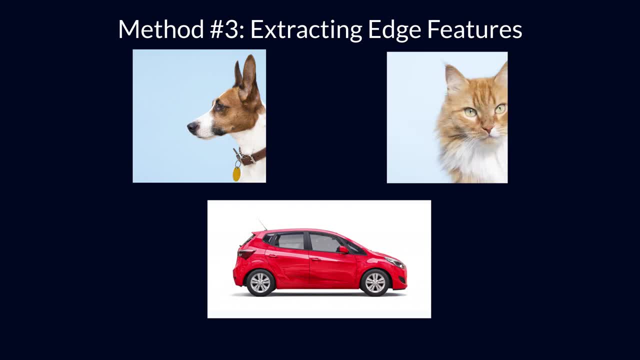 the image and we need to identify the objects present in it. As a human, we easily have recognized the objects in an instant: a dog, a car and a cat. What are the features that you considered while differentiating each of these images? The shape could be one important.